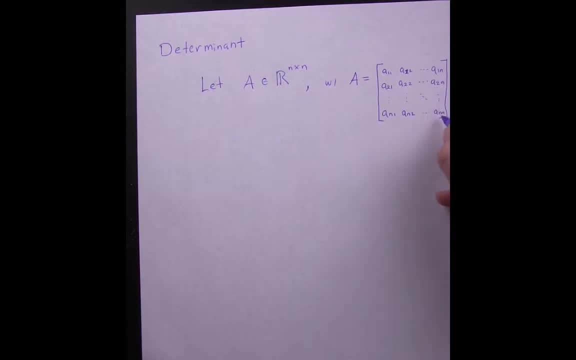 in our definition. So here is an n by n matrix. We define the determinant of this matrix as the determinant of A, to be a sum with n factorial sumands. We're going to talk about this in detail. So we sum over all permutations in the symmetric group on n elements, where 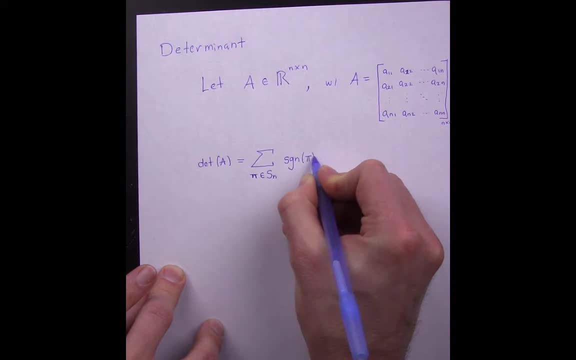 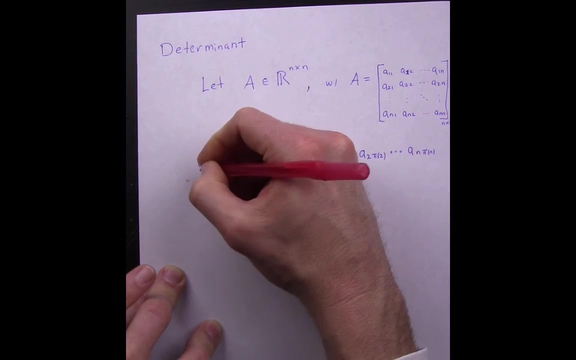 we multiply each sumand by the sine of the permutation, And then the product that follows in between is the product of the individual entries in A, with a slight modification depending on each particular permutation. In this notation this is read: the determinant of matrix A. 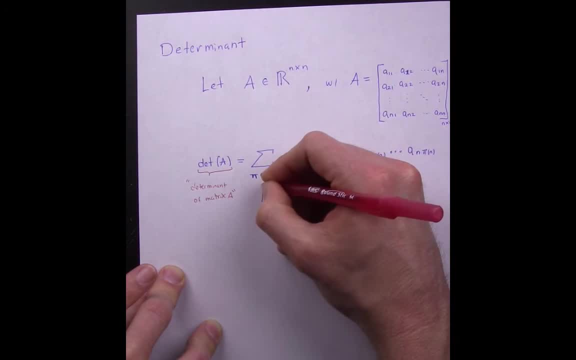 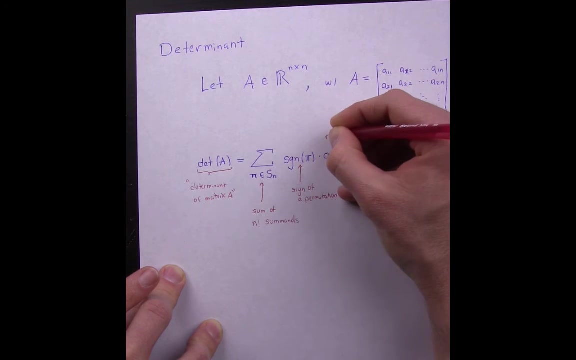 This sum has n factorial sumands, And remember that a sumand is just an individual part of the sum. This is the sign of each permutation. We call this the sign of a permutation. And then here, the first entry we have, this is the row index. So row index 1 corresponds with the first row. 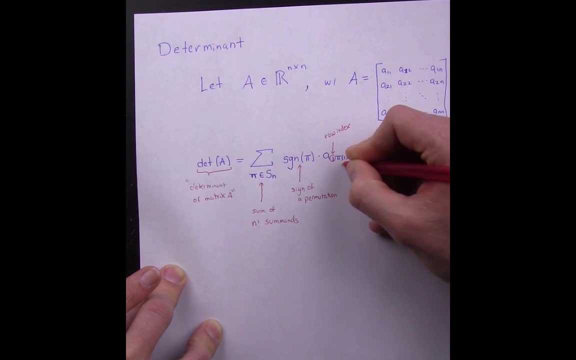 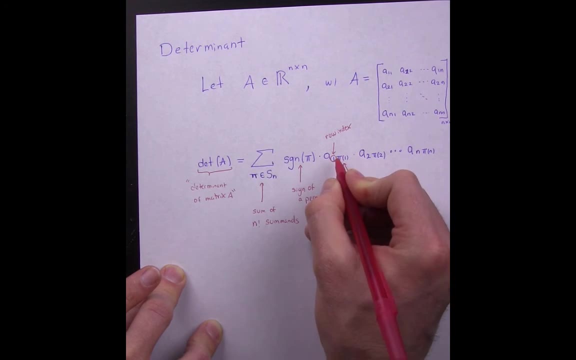 And what happens is the corresponding column index here. this is the column index comes from evaluating the row index through the permutation that we've chosen. So we still have the column index. We start with row 1.. We evaluate 1 at each particular permutation to get 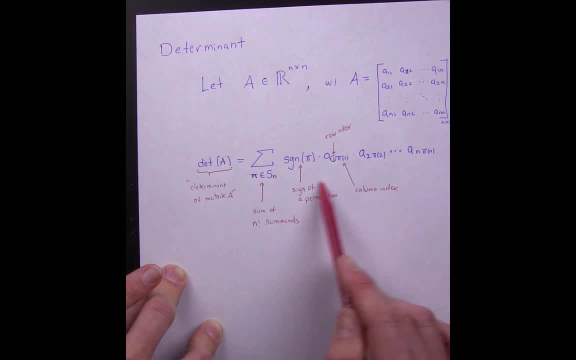 the column index And we go all the way down through n In order to understand this definition of the determinant. we're going to evaluate this for S2, the symmetric group on two elements, and also S3, the symmetric group on three elements. So we will define both permutations for a.